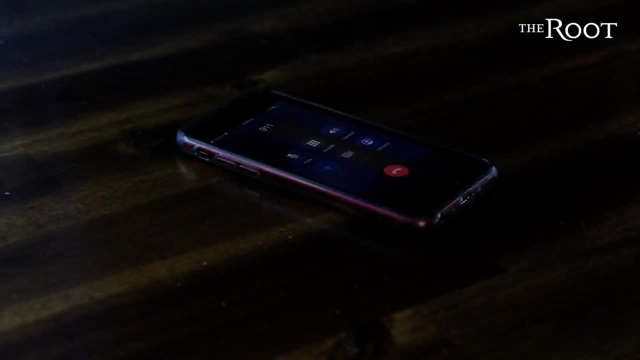 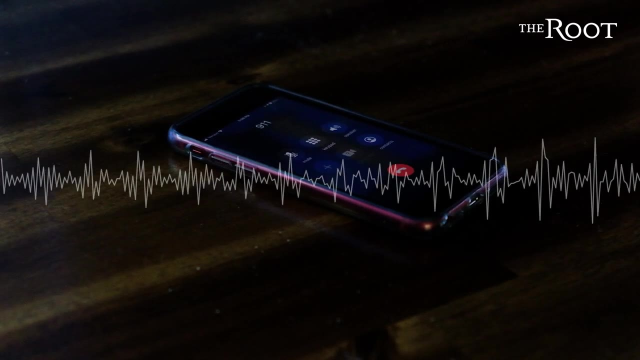 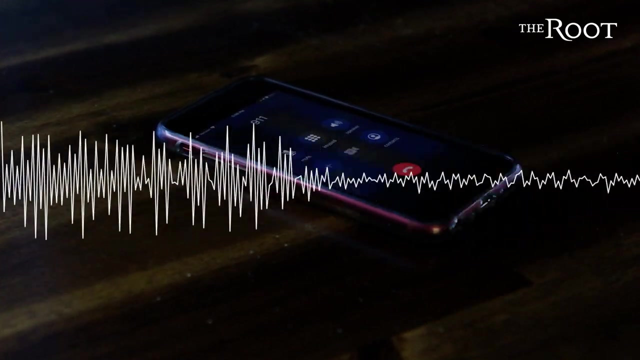 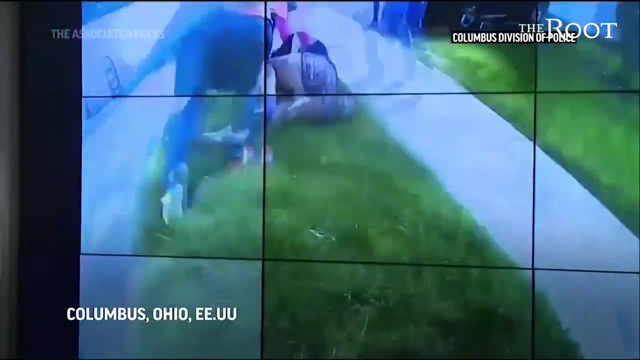 In April 2021, a call was made to the police regarding a dispute at the foster home of 16-year-old Micaiah Bryant. Police arrived at the scene and shot Bryant four times, killing her A Black girl who was defending herself with a knife. What does the chaos leading up to the shooting death? 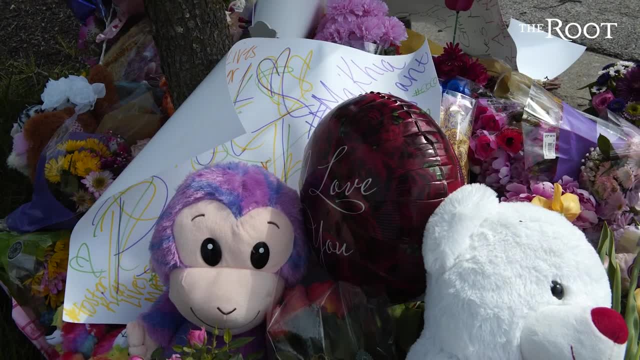 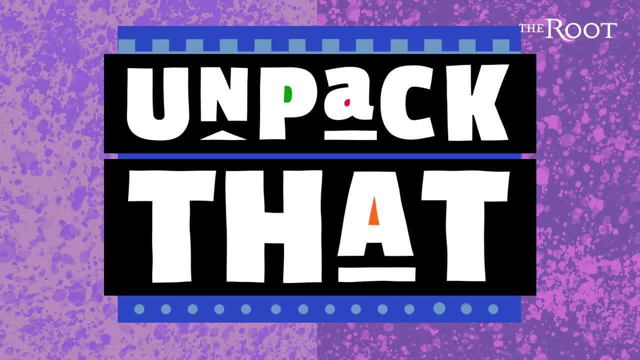 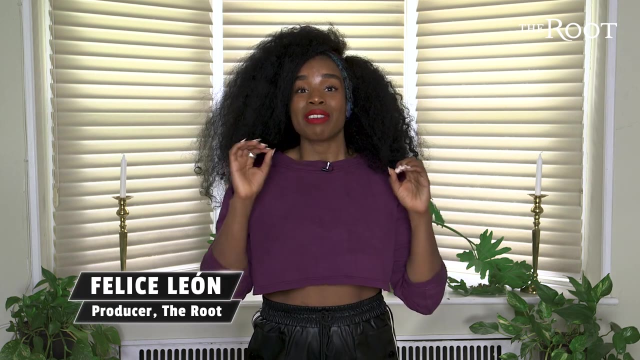 of Micaiah Bryant tell us about Black kids in the welfare system, Today's baggage, how foster care fails. Black kids- The child welfare system is a set of services that support children and families to make sure that they have a safe and adequate space to live and 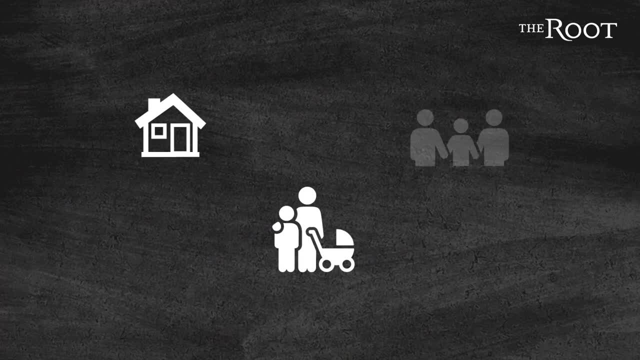 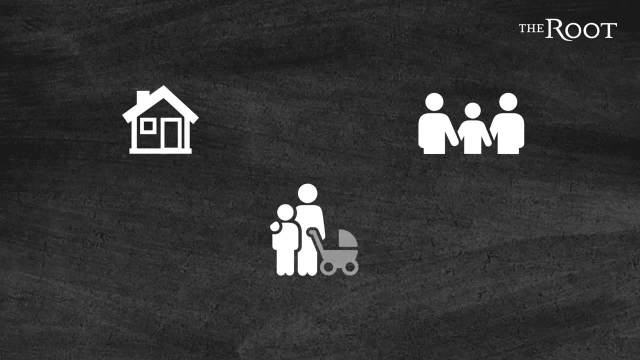 grow Well. supposedly, Child welfare consists of programs like housing assistance, parenting skills classes and foster care, which sets up a system that allows children to live and grow, A system where children can be separated from parents that are deemed unfit Hollywood has. 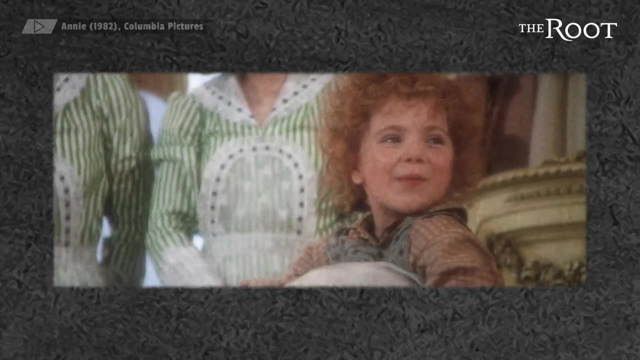 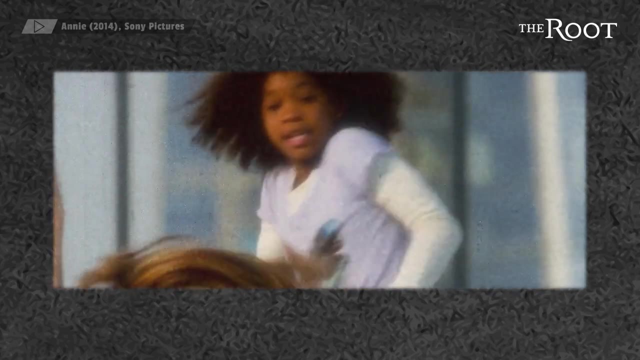 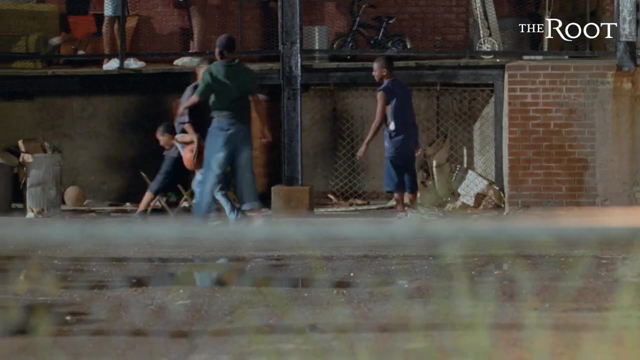 glorified the experiences of kids in foster care with multiple iterations of Orphan Annie. But unlike my Forever Annie portrayed by Quvenzhané Wallace, the reality is that most Black kids in the system don't have that fairy tale ending. In 2018, Black children represented 14% of the kids. 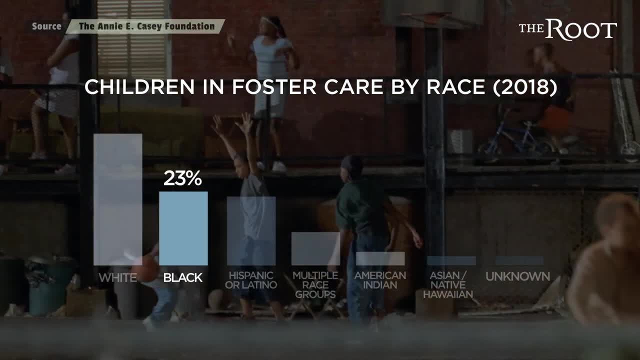 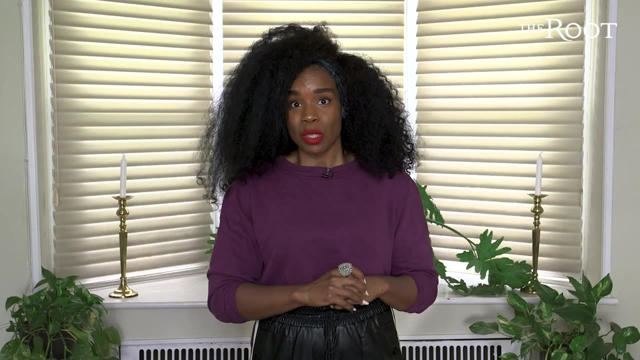 in the US, but 23% of all kids in foster care And just like so much else in this country. in order to get an idea of exactly how the child welfare system got this way, we've got to take it back. 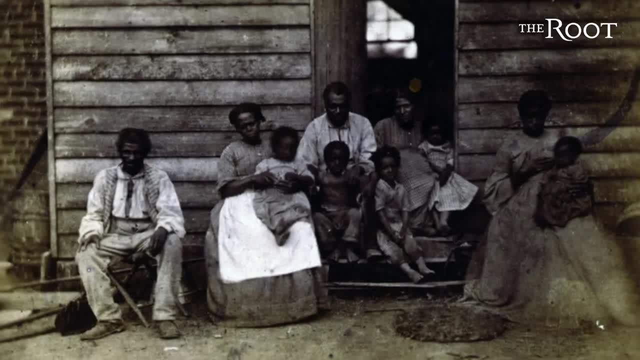 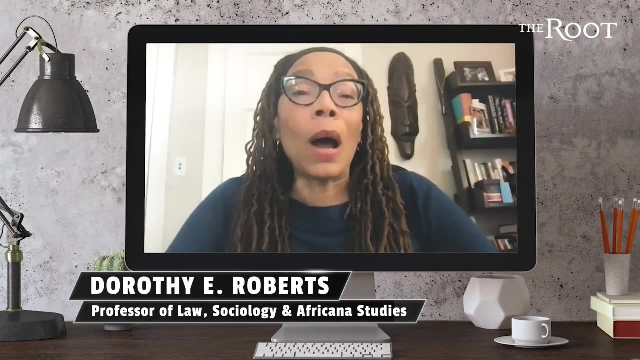 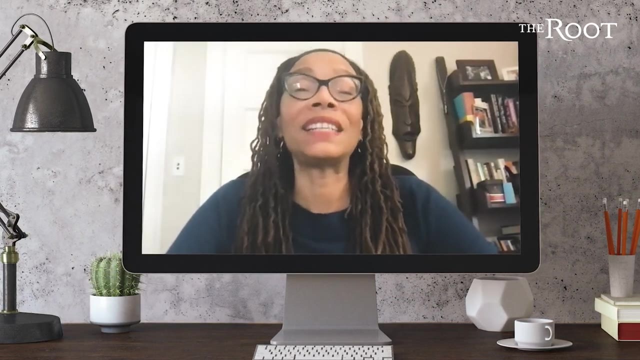 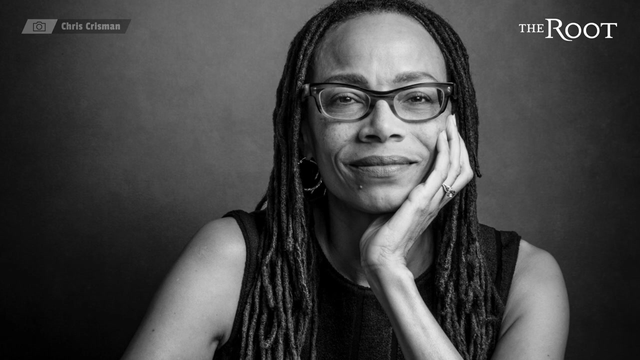 I start by going all the way back to slavery and the enslavement of Black families in the United States, because during that system, White enslavers put themselves in the position of being in control of the entire plantation family, which included Black parents. Dorothy Roberts is a professor of law, Africana studies and sociology at the University of 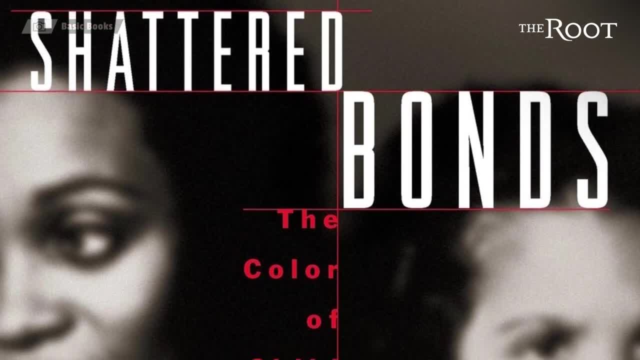 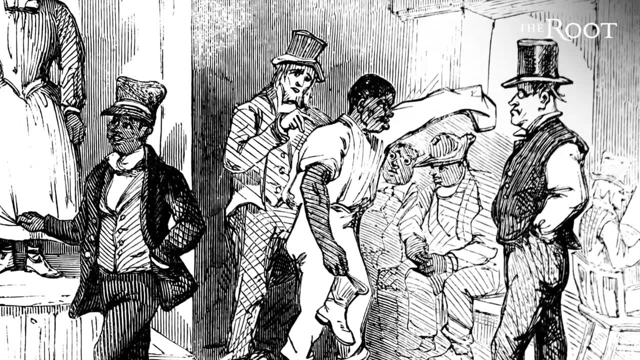 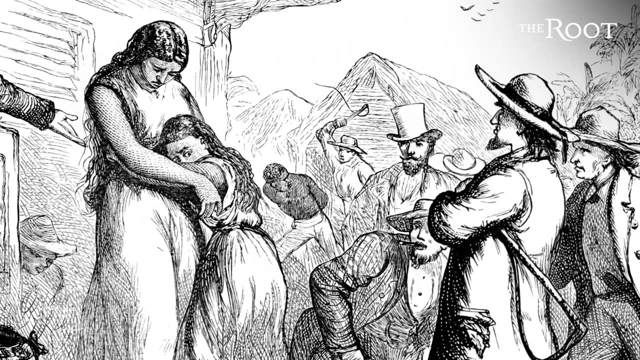 Pennsylvania Roberts is also the author of Shattered Bonds, The Color of Child Welfare. On the auction block, families were often put up for sale and children sold off to other enslavers, separate from the mothers and fathers, And even after emancipation, the separation of Black families was still a thing Take. 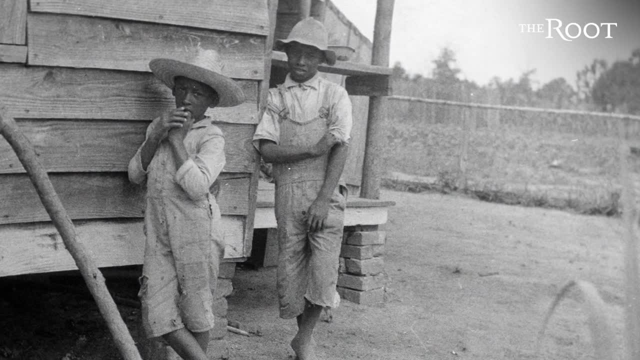 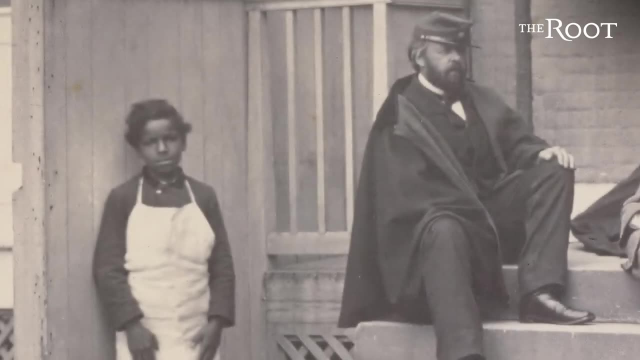 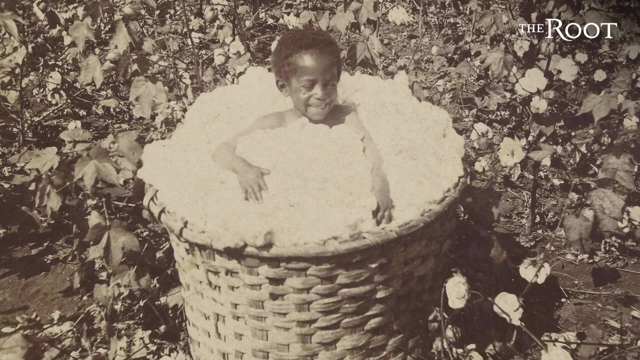 a look at a printout. In this practice, kids were sent away to work for other families. There was rampant apprenticeship of Black children by courts who gave these children over, sometimes to their former enslavers. This was very common And this cruel system of separating children from their families has harmed multiple communities. 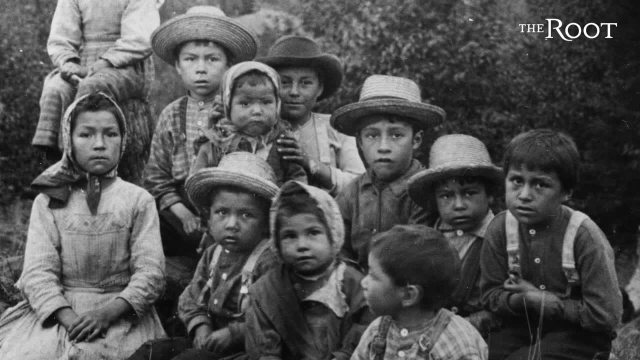 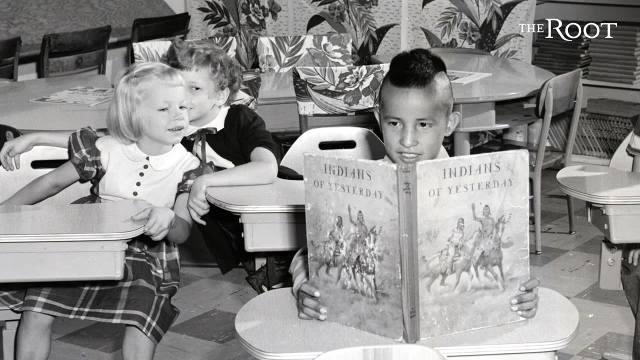 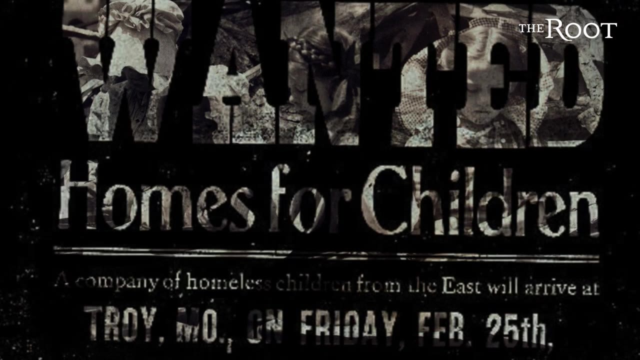 throughout history. In the 1800s, the US government took thousands of Indigenous youth from their families as a form of psychological warfare, Putting the kids in boarding schools with the intention of whitewashing them. Roberts also notes orphan trains as a significant forerunner to our current child welfare system. 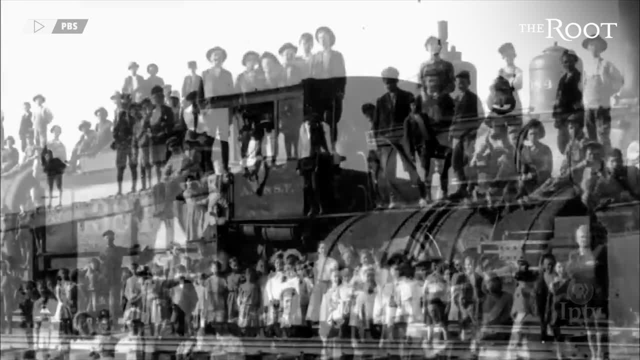 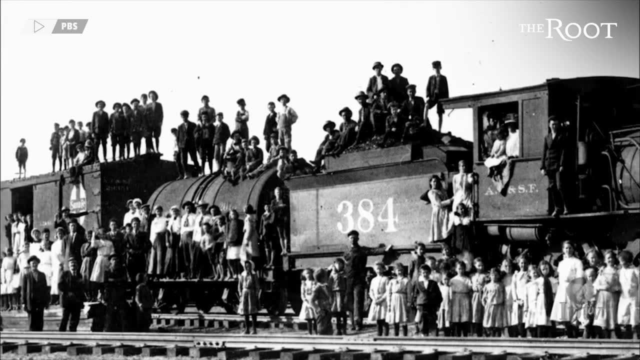 This practice sent hundreds of thousands of homeless, poor white immigrant children from major cities like New York to the Midwest to work on farms in exchange for room and board. In the early 20th century, the federal government finally decided that it wanted to save the 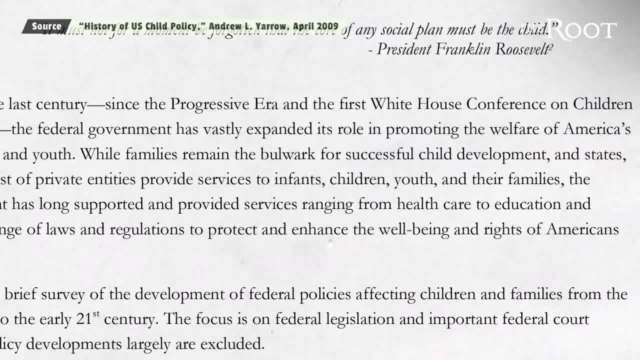 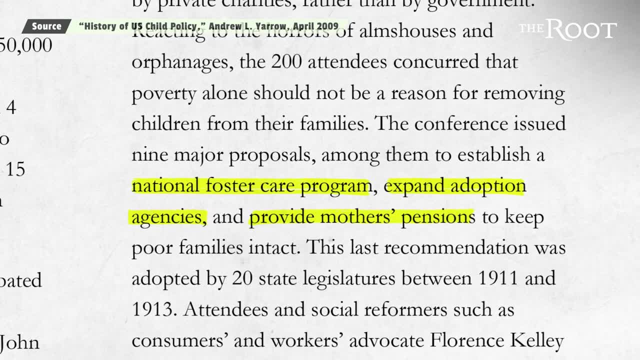 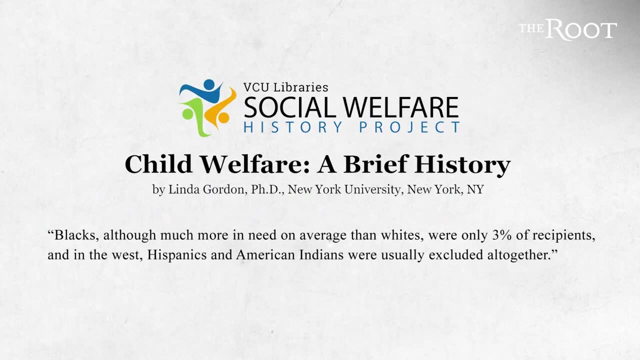 children. The first federal proposals were instituting a national foster care system, expanding adoption agencies and providing monetary aid through mothers' pensions to keep these families intact. The mothers' pensions were for white widows or white women without husbands. Black women were left high and dry from the greater child welfare movement until the Civil 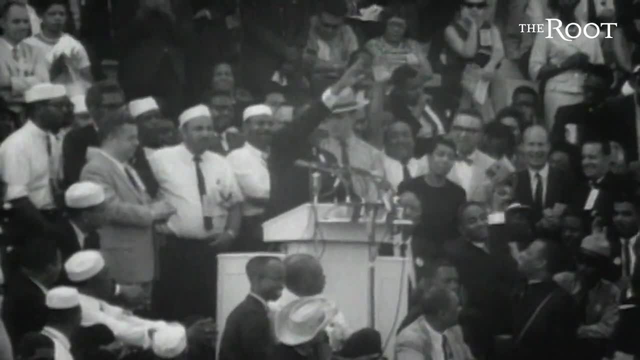 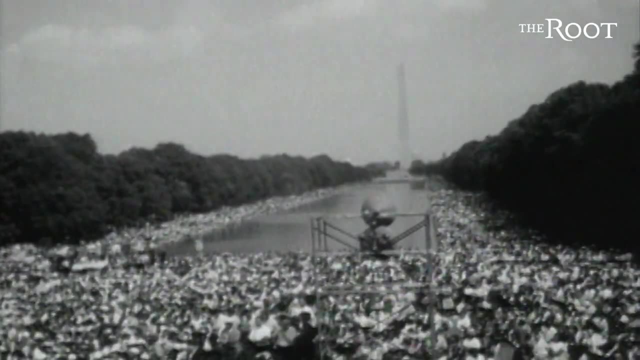 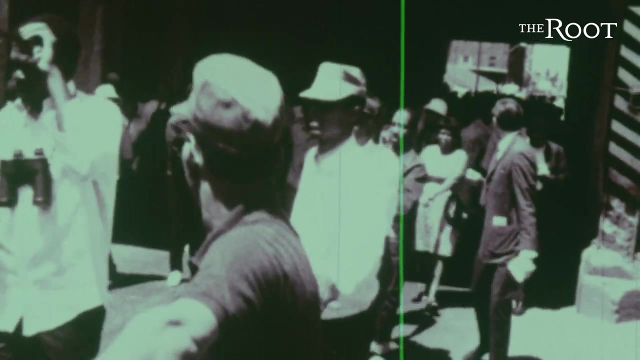 Rights Movement that is Free at last. Thank God, Almighty, we are free at last. Part of the Civil Rights Movement was to extend social welfare, which included Social Security, you know, and Medicaid and Medicare and other kinds of public benefits to support families. 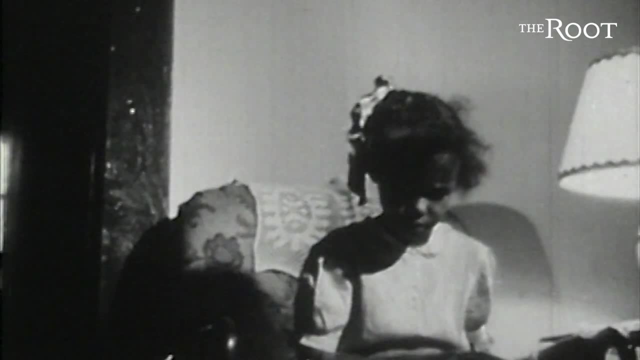 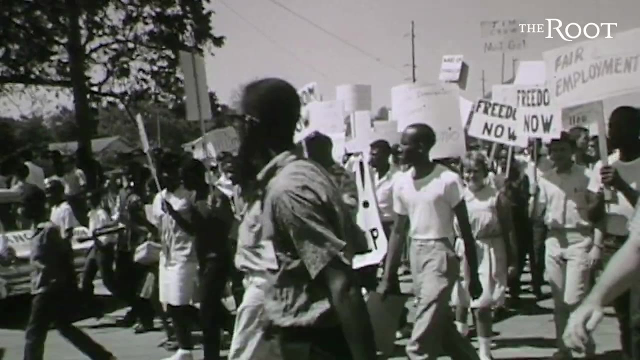 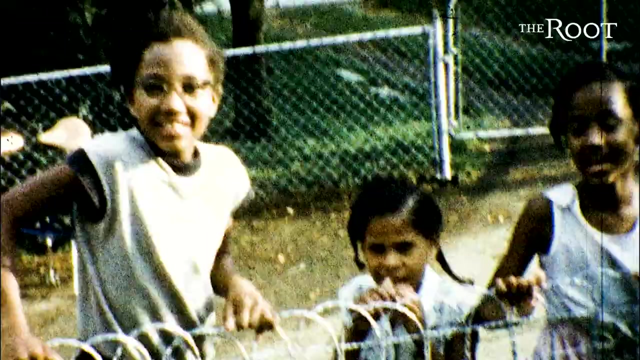 from which Black people had been excluded, And so what happens is, when Black families began to be included in child welfare services, these programs began to become much more punitive. As Black kids were folded into the child welfare system in the 1950s and 60s, more money was. 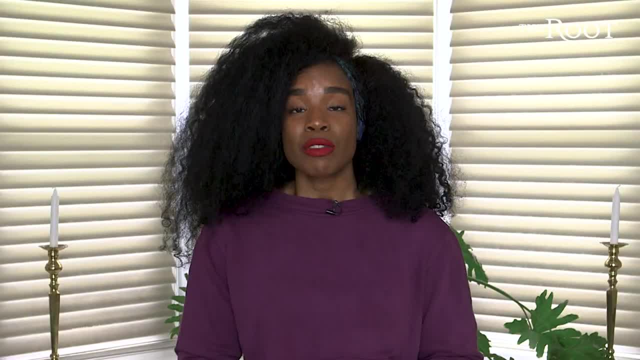 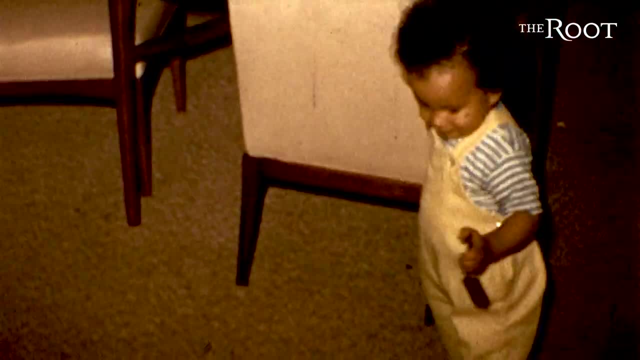 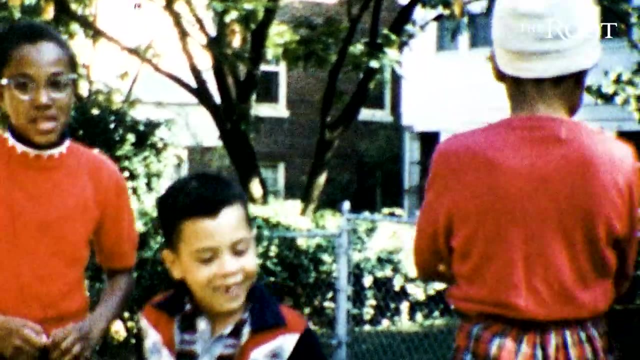 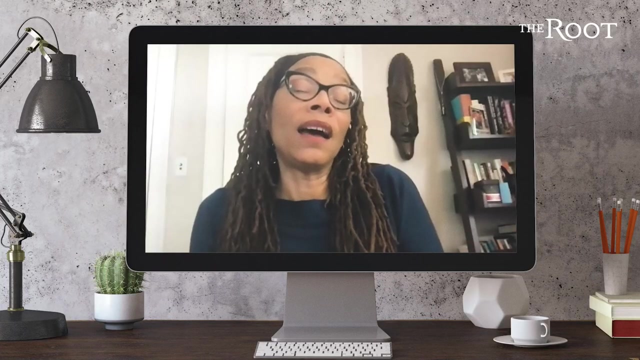 designated to foster care, which by nature breaks families apart. What happens as more and more Black children enter the child welfare roles is that foster care becomes the major so-called service, And we see an explosion of the foster care population simultaneously with this development. 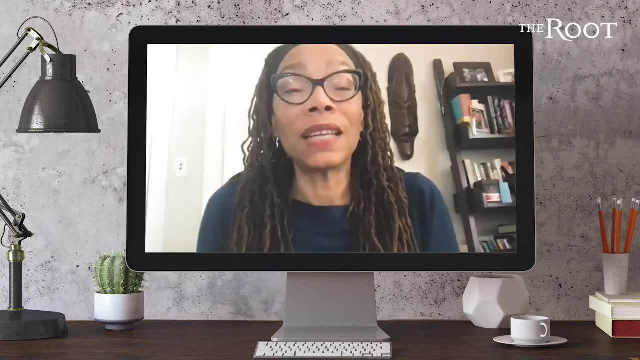 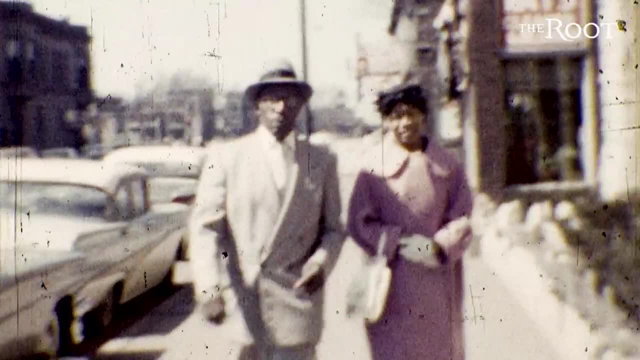 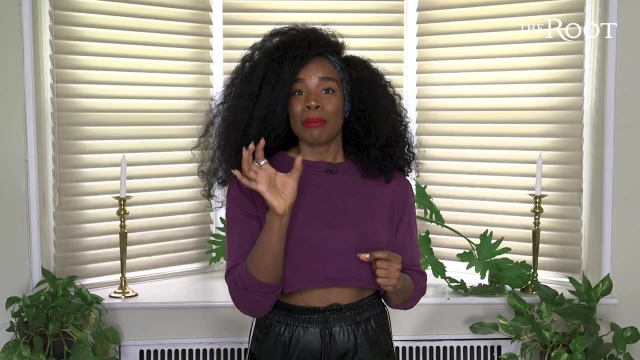 of stingier, more stigmatized welfare benefits up to the basic abolition of the federal entitlement to welfare. So social programs that were once used to support white families are now used to control Black families, And those same programs disproportionately regulate and investigate Black families too. 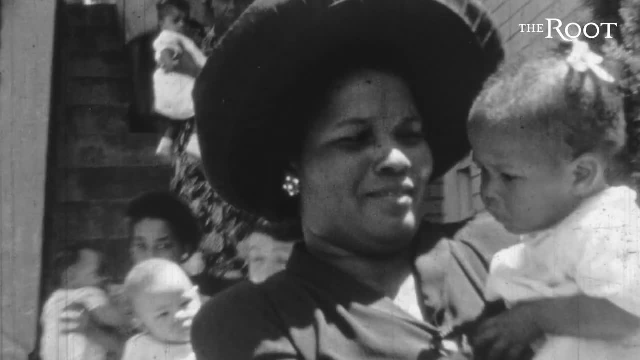 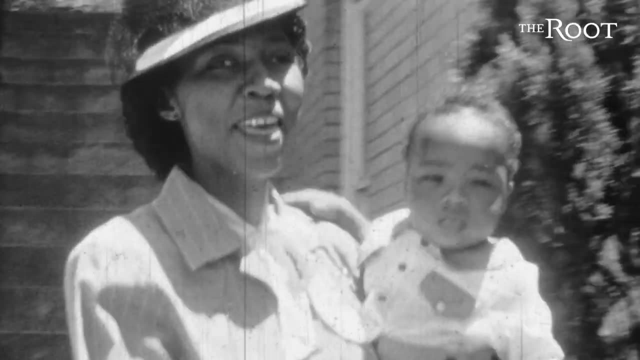 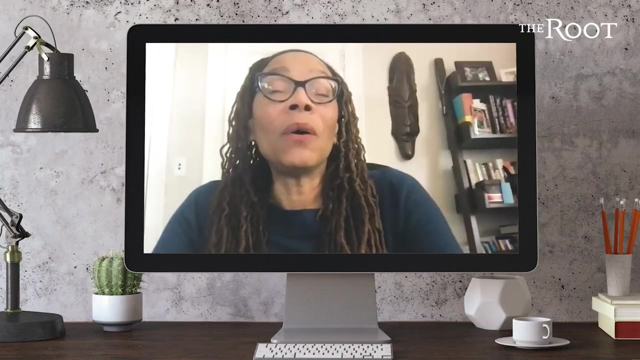 Robert says that part of this disparity is due to the racist ideology that Black mothers were harming their children, And this damaging and problematic way of thinking is a weapon still being used against Black parents and families today. We can go back to slavery as the origins of this idea that white people need to save Black 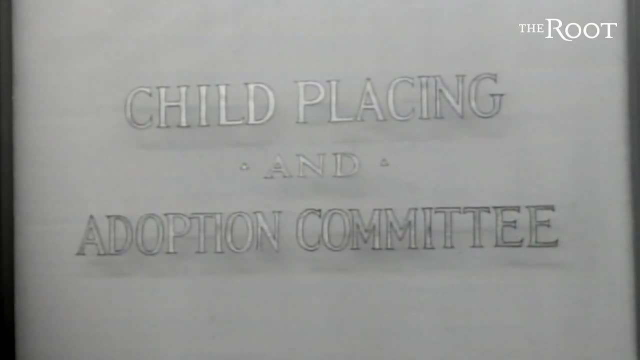 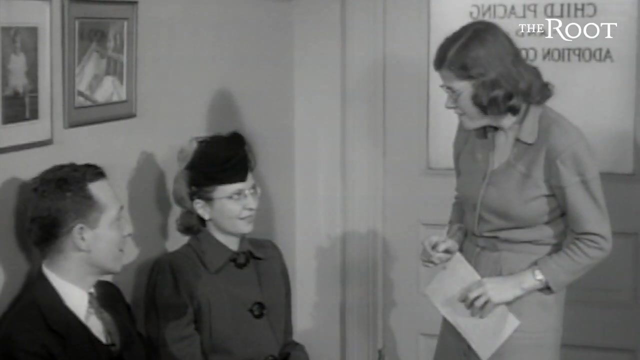 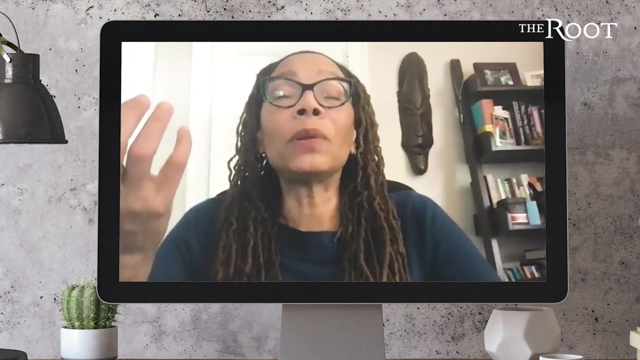 children from their families. And from the beginning it's been not only a false but a racist, white supremacist ideology that paints Black parents and families and communities As if they're defective and harmful, And so it really twists completely. you know, in the opposite direction, what the child welfare 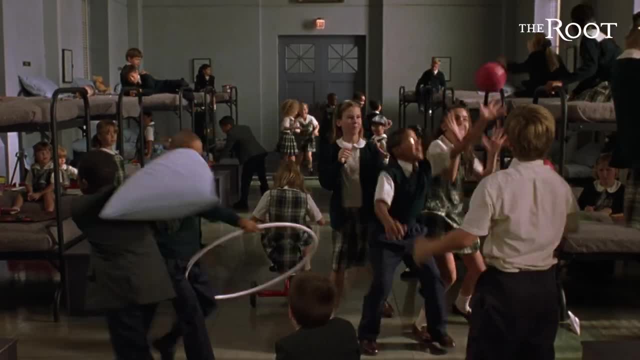 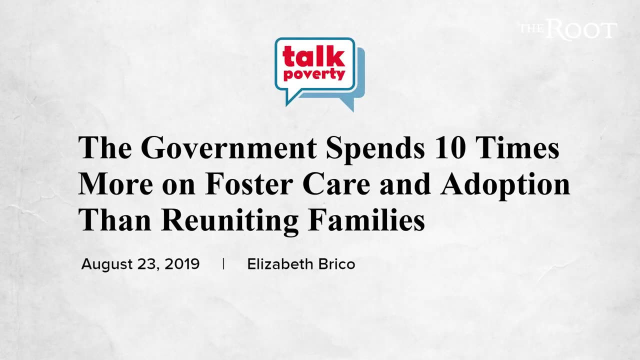 system is really about. Rather than being proactive, child welfare has become reactive. The federal government spends 10 times as much money on foster care as it does on reunification, And let's not even start to discuss the preventative services that could be used to prevent children. 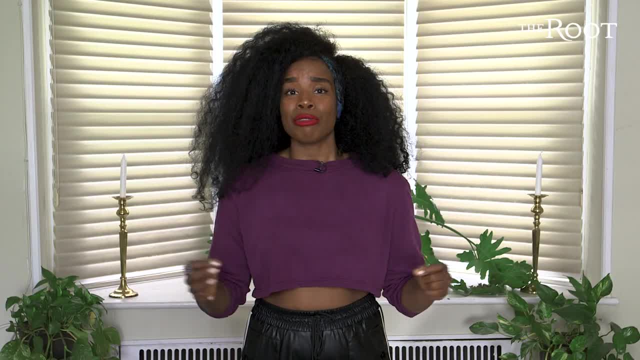 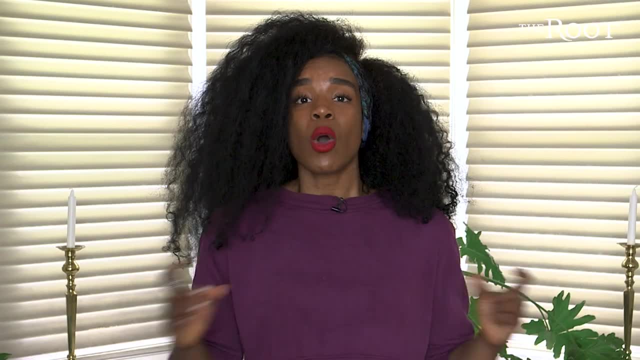 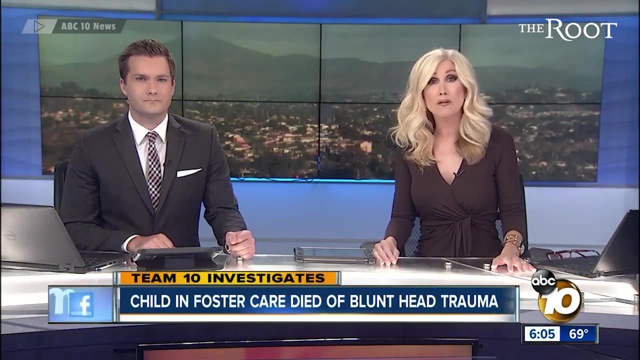 from entering foster care in the first place, And if we really don't want to traumatize kids, then perhaps we should be considering programs aside from foster care, Because, by all accounts, foster care is grim. There are questions about the death of a child who was in San Diego County foster care. 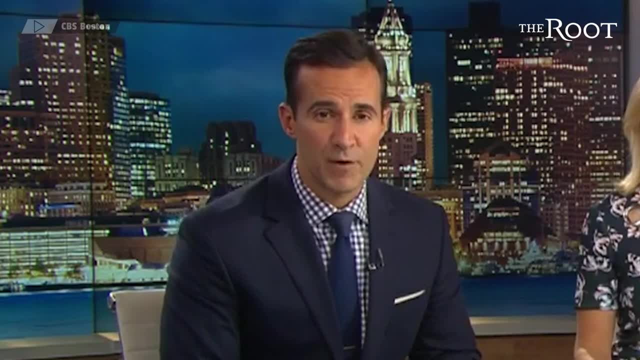 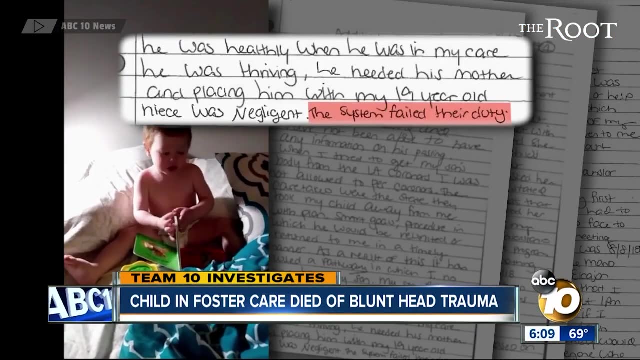 The child's grandmother tells WBZ's I-Team that the system failed that girl. There's lots of studies that show all the bad outcomes for children in foster care. They're more likely to be incarcerated, to be in juvenile detention, less likely to go. 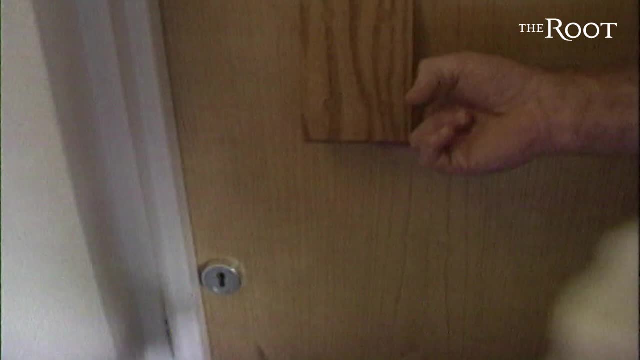 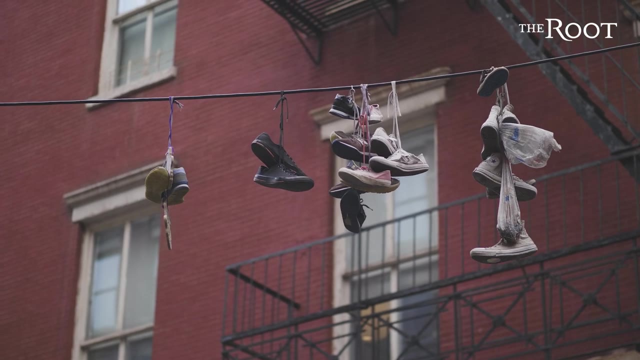 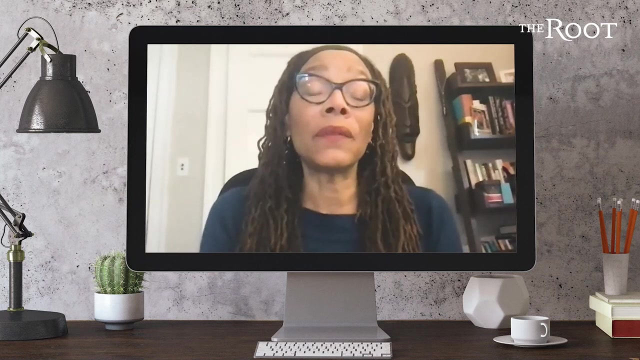 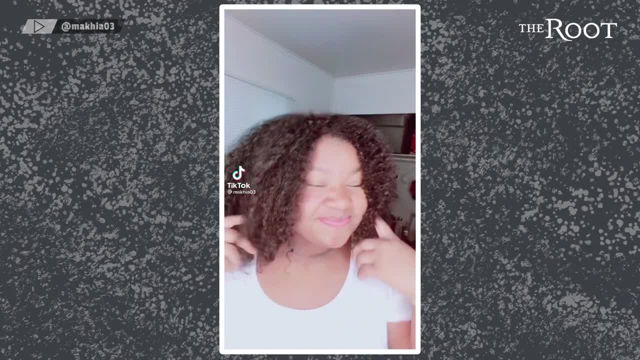 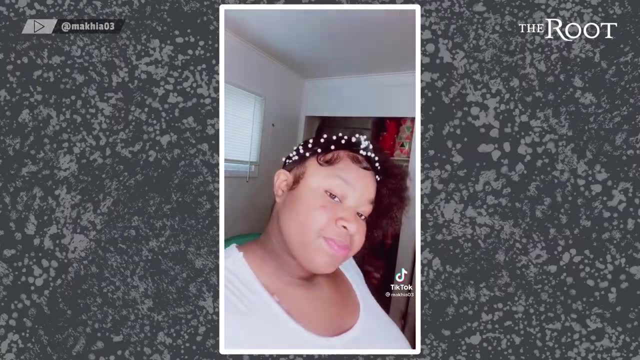 the whole system is structured. Micaiah Bryant was a 16-year-old who laid her edges on TikTok. like many young Black girls, She was a sister and a daughter and a friend, but ultimately was a Black teenager who was entangled in the child welfare system. 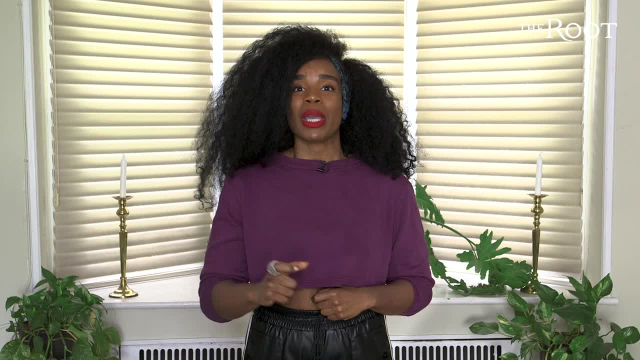 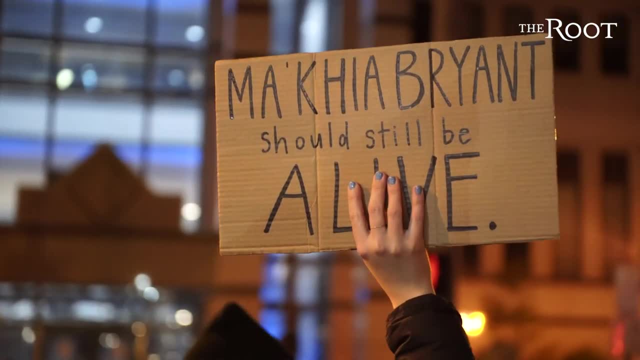 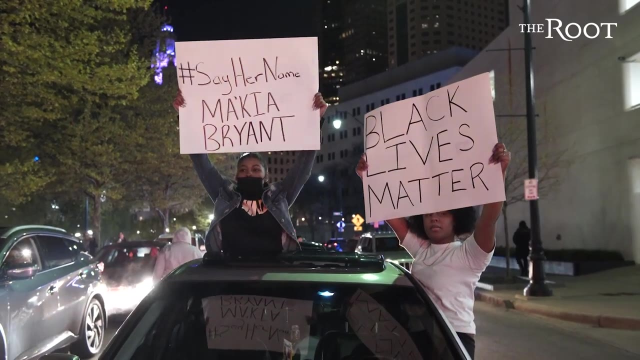 How does Micaiah Bryant, being a Black girl in foster care, shape the way that we understand the tragedy that is happening? We have to ask why she was in foster care and the conditions of foster care. Many Black children, especially teenagers, are put in congregate types of care where 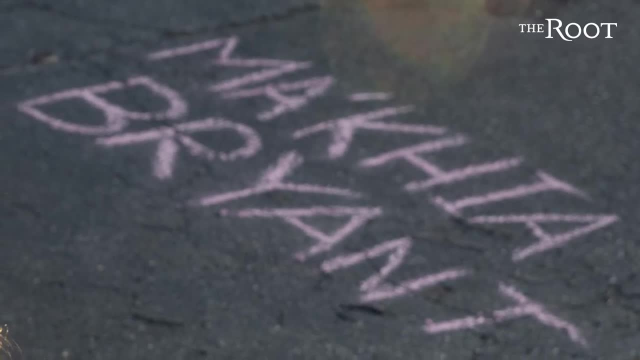 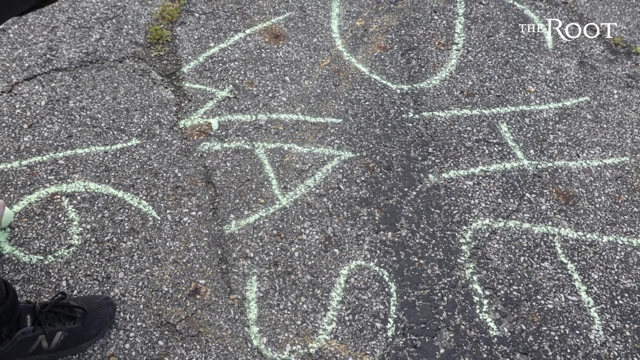 there are lots of children who have been put together in traumatizing and stressful situations. If you are thrown together with a child who is in foster care, you are not going to be able to get out of the foster care system. If you are thrown together with a child who is in foster care, you are not going to get 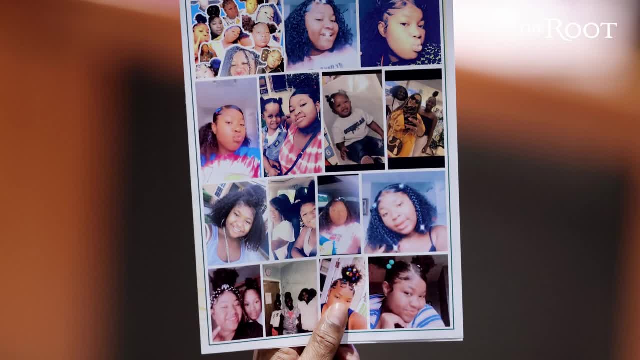 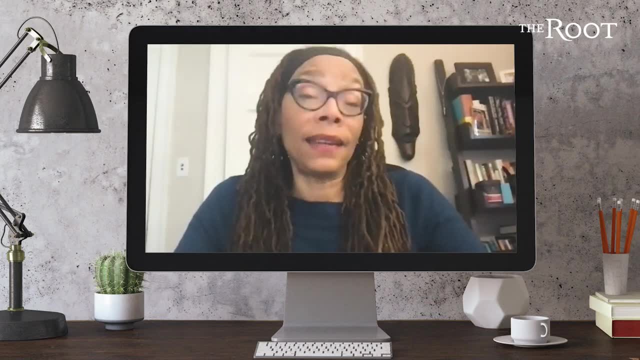 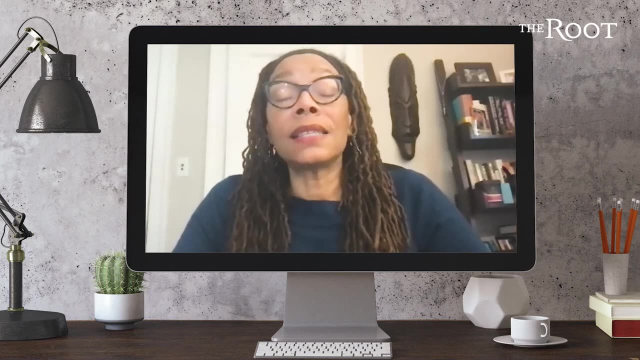 out of the foster care system. If you are thrown together with other teens and adolescents who have been taken from their families, it's not surprising that there would be a fight between children in foster care. It happens all the time And in many of the cases law enforcement is called in. 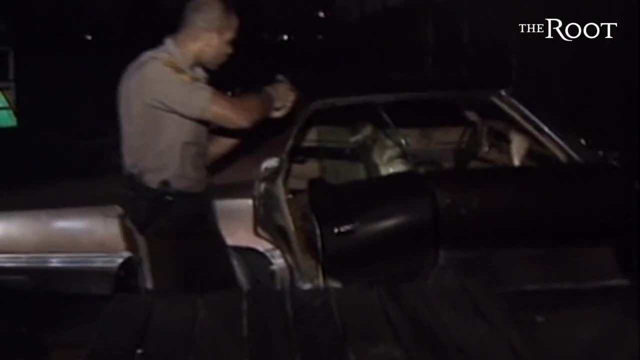 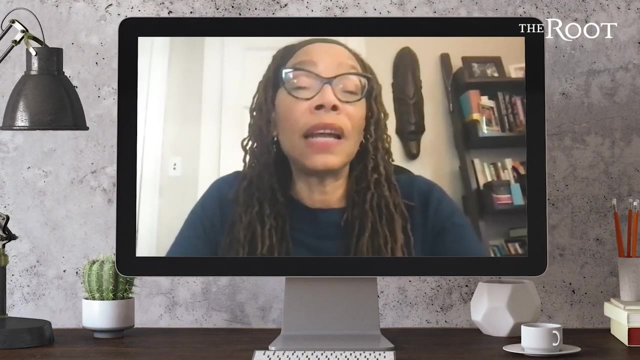 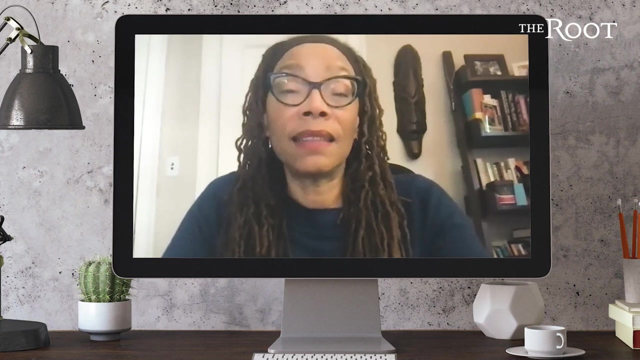 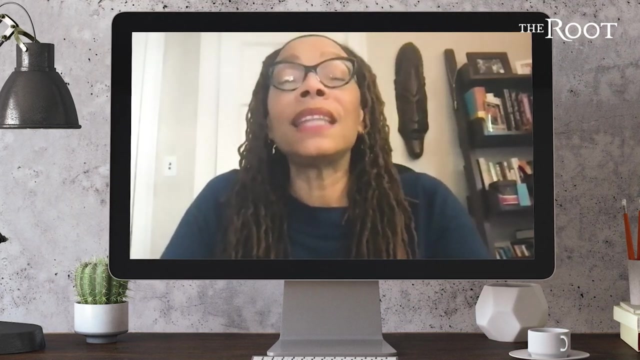 Black children in America are already at higher risk of having encounters with law enforcement, being arrested, being detained, In fact, being imprisoned as adults. So when you add to that the way in which foster care makes them even more vulnerable, that makes their situation worse than that of white children. 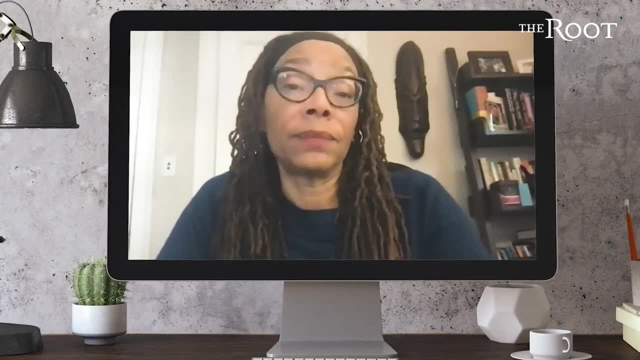 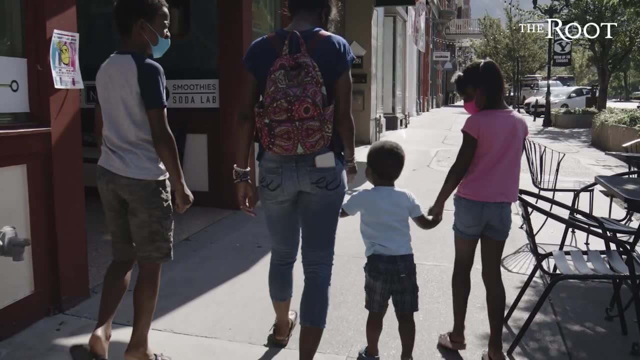 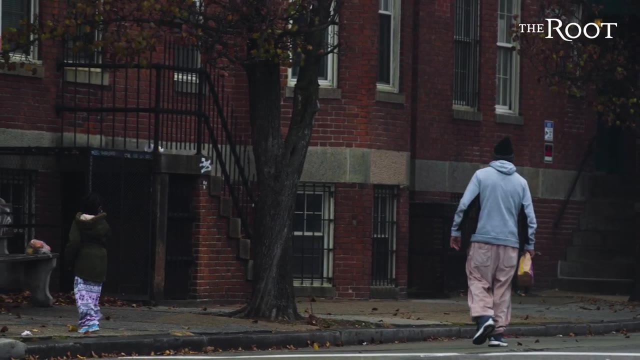 Structural racism and racial biases in child welfare increase the likelihood that Black families will be separated. While in some cases this does protect children, many children have become vulnerable to violence, including to child abuse. They become the victim Many times. it traumatizes the children who have become a part of the child welfare system. 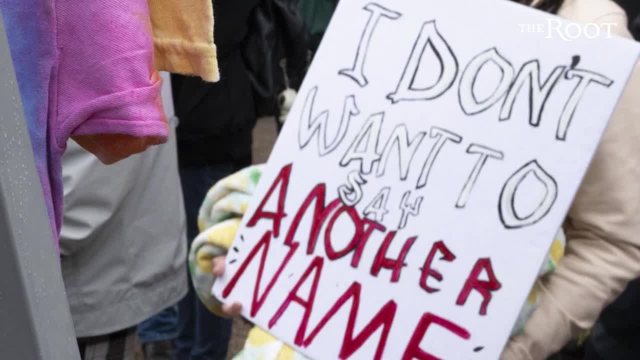 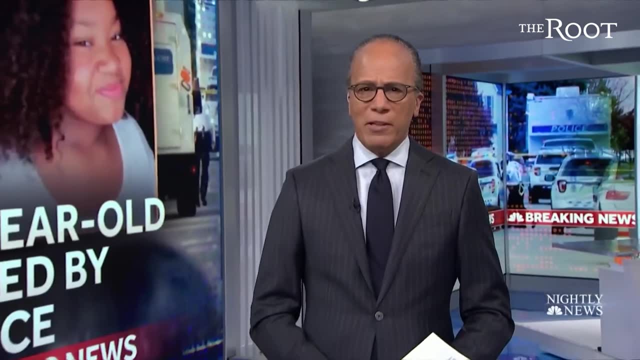 or even puts them in danger. Let there be no ambiguity: Makiya Bryant's death is due to multiple failures in the American system, from policing to foster care, which put her in a situation where she had to defend herself with a knife. 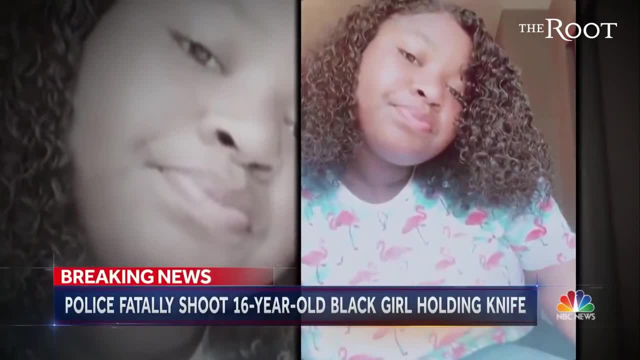 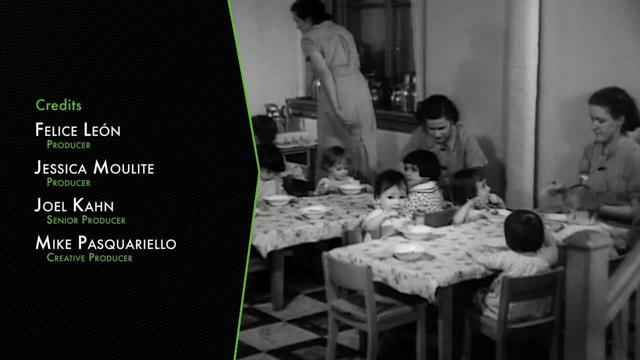 While child welfare and foster care literally break families apart, it isn't hyperbolic to say that the child welfare system itself is broken. Welfare workers are trained to treat each child as an individual. Every effort is made to duplicate a normal, happy home life. 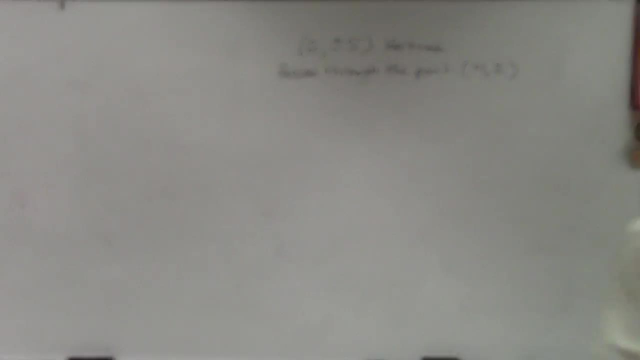 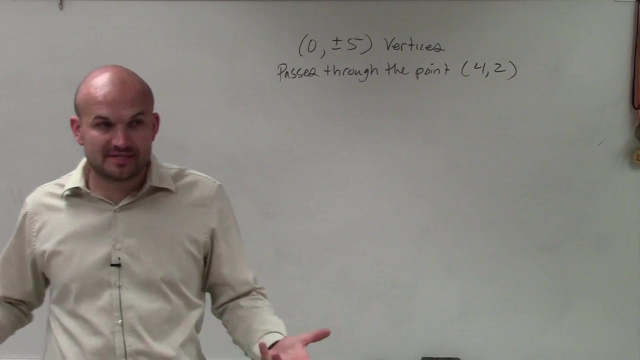 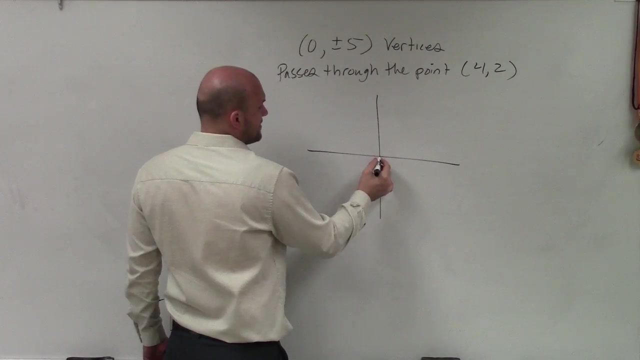 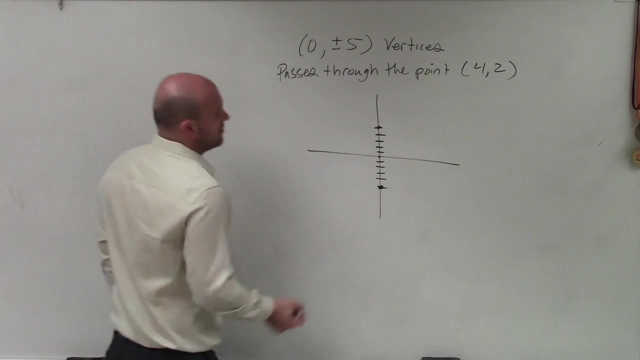 Okay. so on this one again, guys, before I'm going to be doing anything, before I want to do anything, I got to be able to determine what type of equation am I going to be dealing with. So let's plot the information that we have. It says: my vertices are: 0,, 5, and 0, negative, 5. 0,, 1,, 2,, 3,, 4,, 5.. 0, negative: 5. 1,, 2,, 3,, 4,, 5.. Verticy- verticy, Since my vertices all lie on the 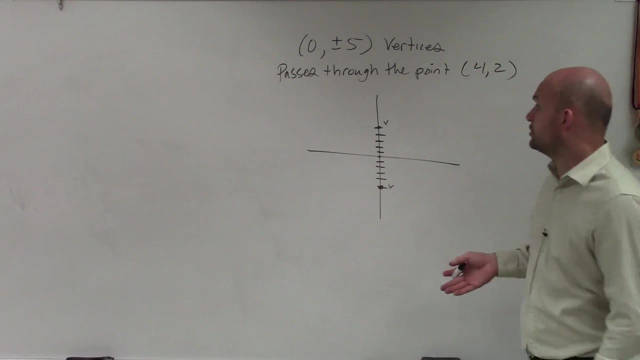 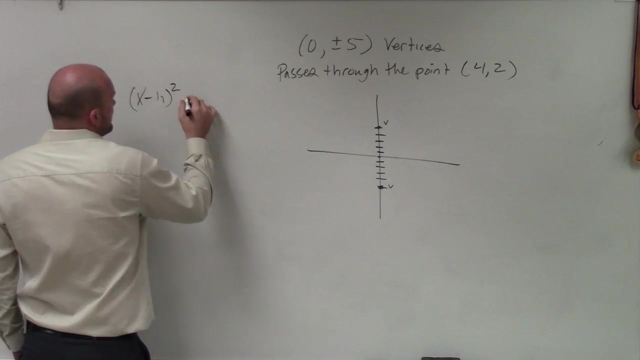 same major axis. is that major axis going to be vertical or horizontal? Kaylee, Vertical right. So that means there's only one equation that I can use. That's the one for a vertical ellipse. So that's x minus h squared, plus y minus k squared, And then here it's going to be b squared over a squared. where now the value of my a, the distance? 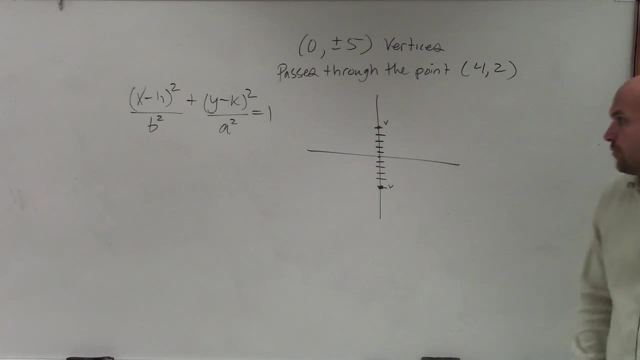 squared of my vertices to the center is going to be under y. So remember, if here's my two vertices, here's my center Right, And that's good. And also, since we know the distance, we can determine that the distance from the center to a.